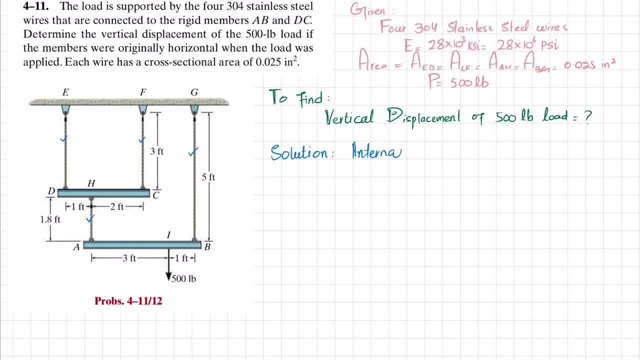 So internal forces in wire. So what we will do? we will take free body diagram, FBD for AB. What is AB? AB is this rigid bar. So I will draw this bar AB Clear. Let this is AB. So at this point B we have a load of FBG. 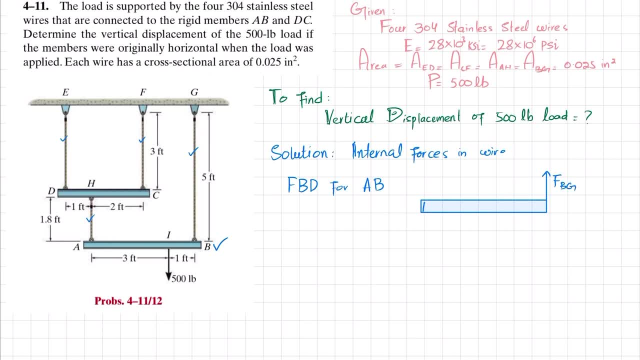 FBG. At point A we have a load of FAH. By drawing this line of AD, which is equal to AB as long asっちゃN number, and there is a load of 500 pound. So that will act به combined and the distance from this. 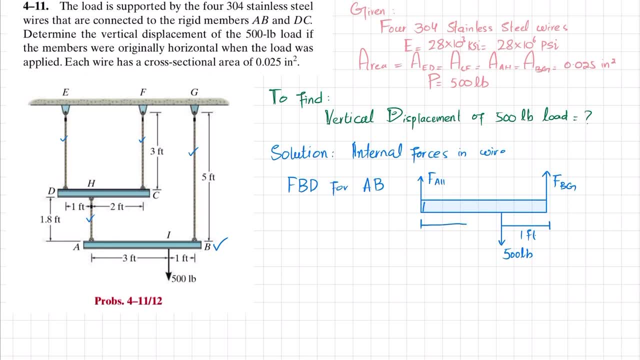 to point B is given as one feet, while this distance is given as 3 feet. I will show you over here. we can see point b and this is your point i. okay, so we will. we will find this. unknown forces f a h and f b g. 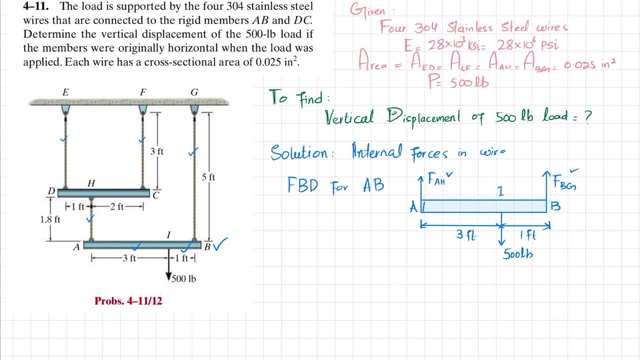 by using equilibrium condition. so what we will do is that we will apply equilibrium condition. sum of all moment about point a is equal to zero and taking the counterclockwise moment as positive, now at point a, one moment is due to 500 and perpendicular distance is three feet and it. 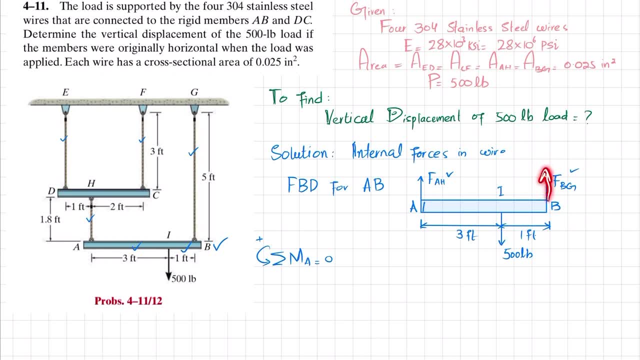 will be clockwise. the other moment is f b g and perpendicular distance is this: total four feet, and it will be counterclockwise. their sum must be equal to zero. so four feet into f b g, that is counterclockwise. f b g minus f a h, not f a h. we are taking moment about point a minus 500 into three is equal to: 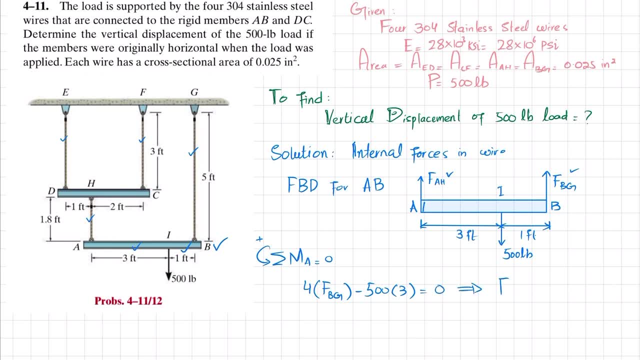 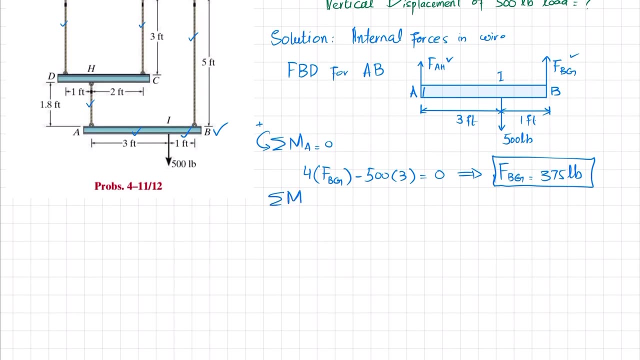 zero. so from here you will get f, b, g will be equal to 375 pounds. now you have this 375 pounds, you will apply another equilibrium condition that sum of all moment are. you can now simply apply this equation: that sum of all forces along y direction must be equal to zero, and taking the upward force as positive. so there are three forces. 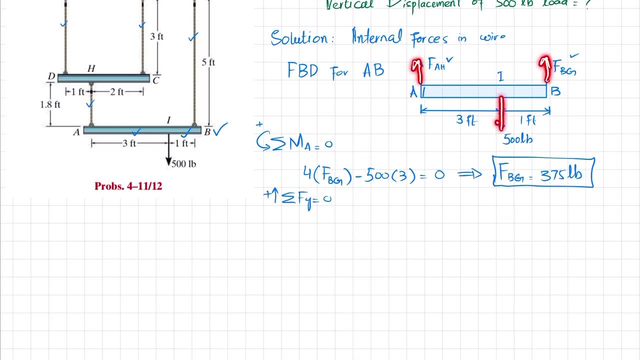 one is this upward, the other one is this upward and lower one is downward. their sum must be equal to zero. so f a h, f a h is positive, plus f b h, which is 375 minus 500, is equal to zero. so from here you will get: f a h is equal to 125 pounds. so these two forces have been calculated. now we will move. 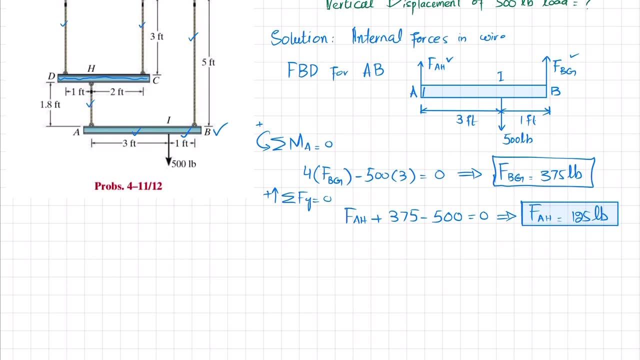 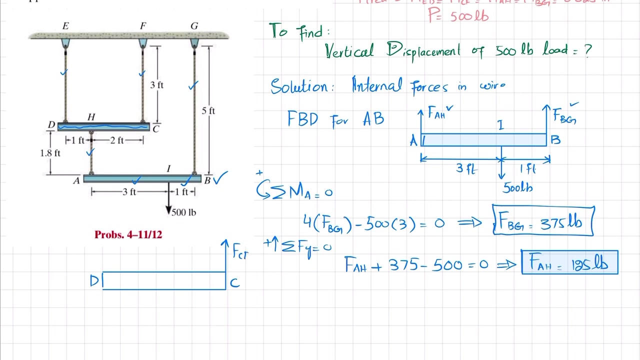 toward member d, c and we will draw the free body diagram over here. so let this is your remember. this is your point d, this is your point c. at c, we have upward force that is represented as f, c, f. at point d, we have a force upward that is f. 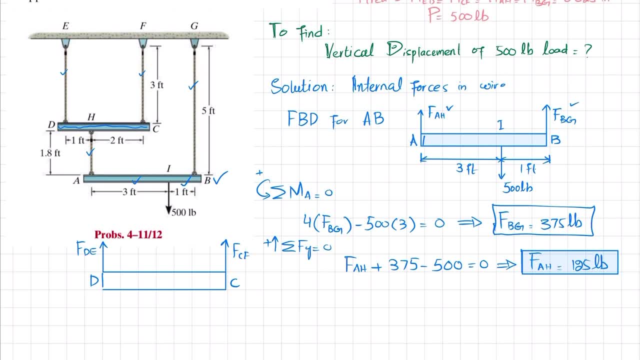 f, d, e and, at this point, h. we have a force that will be now downward and this will be f a h. f a h is in this portion it was opposite and here it is taken as downward clear. also, distance between d to h is one feet and from h to c this distance is two feet. so we will apply equilibrium condition. what 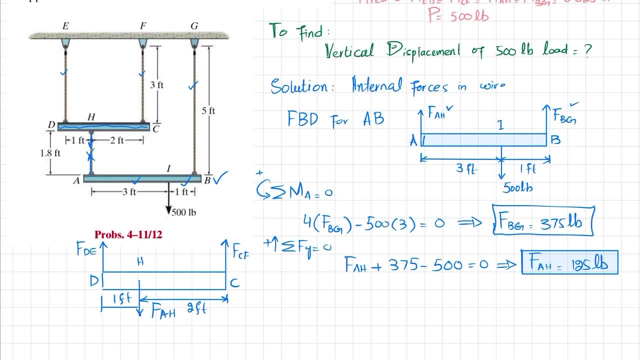 equilibrium condition we will apply. so we will apply equilibrium condition that sum of all moment about point d is equal to zero and taking the counterclockwise moment as positive. so about point d, one moment is f- a- h into perpendicular distance is one feet and that will be clockwise. the second moment is f- c- f into perpendicular distance is three. 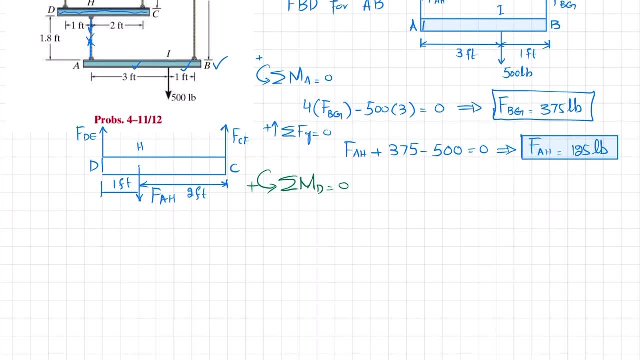 and that will be counterclockwise. okay, so f a h into perpendicular distance is one and that is clock. f a h into moment about point d is equal to into one and that is negative, because this is clockwise. plus f c, f into perpendicular distance is three. there sum must be equal to zero. now you can see f c, f is one to. 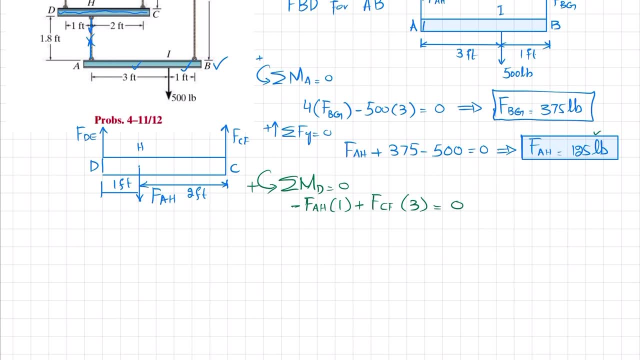 f a, h is one twenty five, clear. so we will write minus one twenty five into one is one twenty five. 3 fcf is equal to 0, so from here you will get: fcf is equal to 41.67 pound. okay, we will apply another equation: that sum of all moment, sorry, sum of all- forces along y. 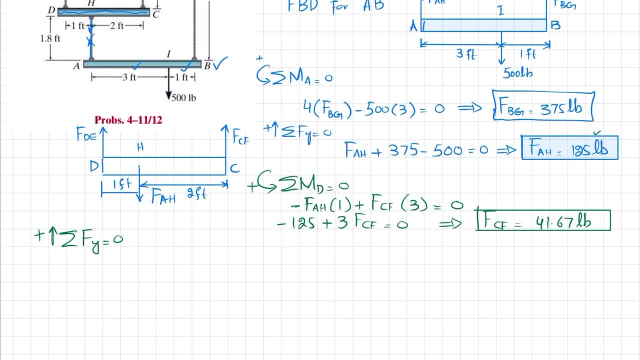 direction must be equal to 0 and taking the upward force as positive. so one force is this, other one is this, and third one is this one. so fde, fde plus fcf, which is uh, which is this: 41.46, 41.67 minus fah, which is 125, their sum must be equal to 0. so from here you will get. 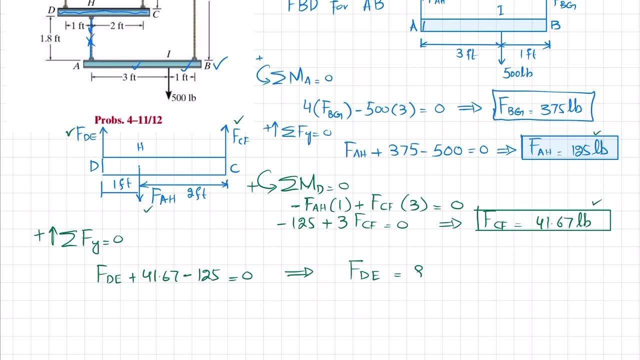 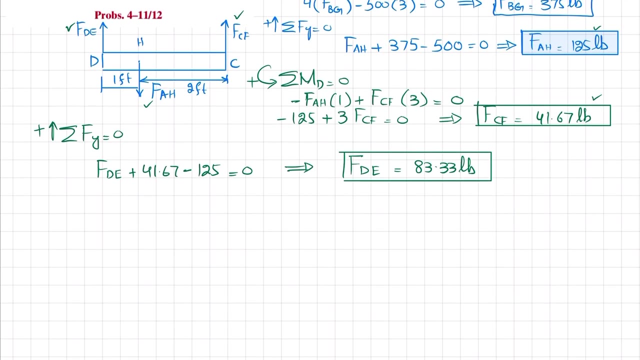 fde will be equal to 83.33 pounds. now we have all the forces in wire in this wire, in this wire, in this wire and this wire, so we will calculate the displacement. so for displacement, displacement, we know that general formula for displacement is equal to f into l, divided by a into l plus. 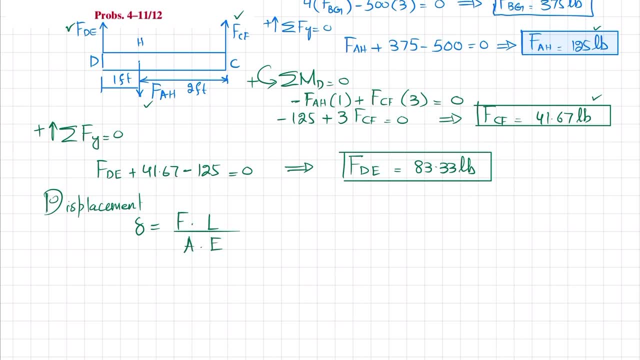 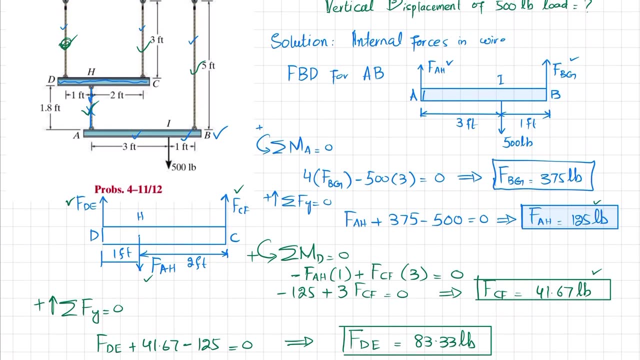 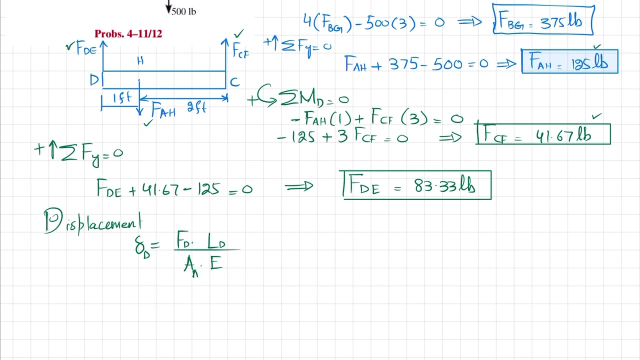 normal formula, fd, which is equal to 1 celebrant plus 5, stepped after那就 into e. so for displacement of point, displacement in wire d in this wire d, so if i write it it will be d, fd, ld, a, d into e, so fd is 83.33 salary. 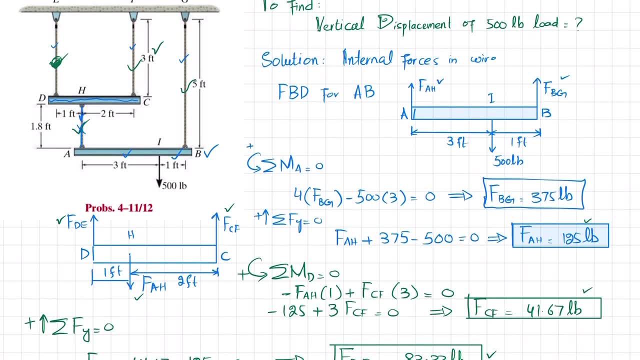 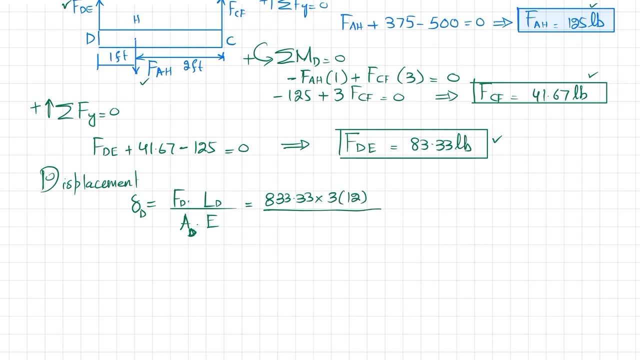 So length you can see it is 3 feet so I will convert it into inch. so 3 feet into 12 will convert it into inch. divided by area of each wire is given as 0.025 and E is 28 into 10 to the power 6 given in the given data. 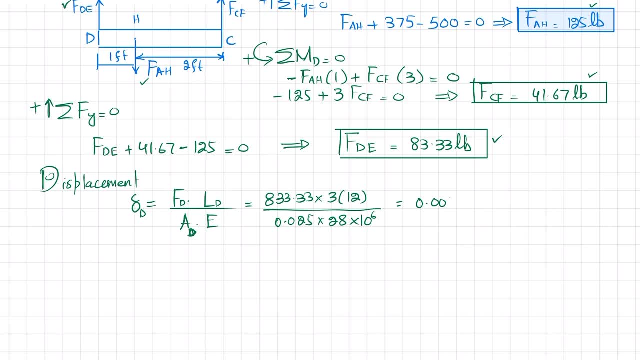 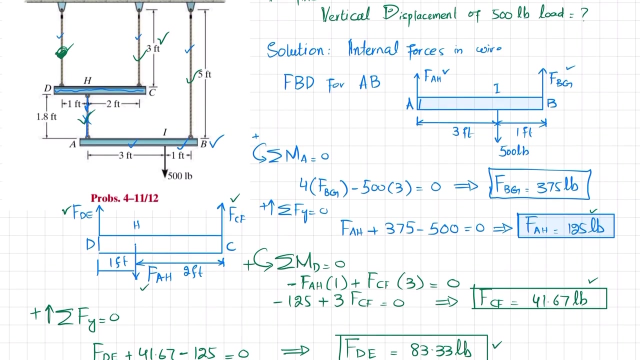 So if you calculate it will be 0.0042857 inch. Similarly, you can also find displacement of point C, that will be FC into LC, divided by AC into E. So FC is generally in this, which is FCF. so FCF is 41 point. 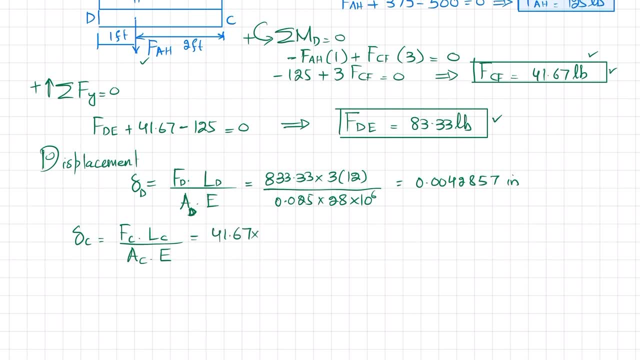 67, so 41.67. length is the same 3 feet, so 3 into 12 will be converted into inch. divided by area is 0.025, multiplied by 28 into 10 to the power 6.. So when you solve this, this will be 0.0021429 inch. 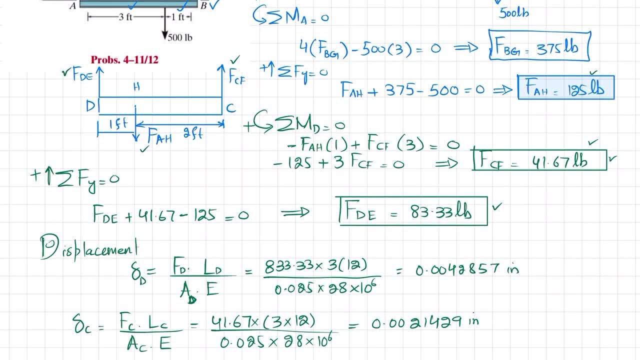 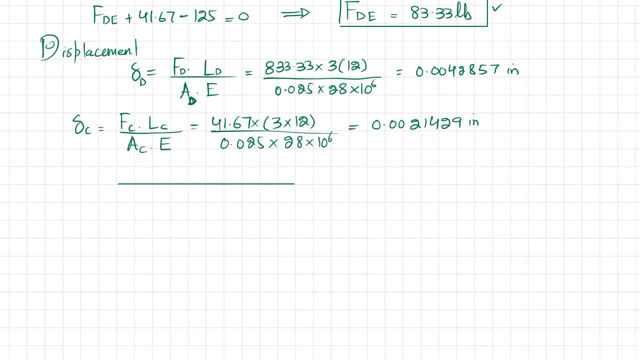 Now you can, if you assume this DEC, DC, DC member. So in Initially it was like this: This is your point D, This is your point C. Now you, after displacement, you can see, point D is let. this is the displacement, This distance is the displacement which is represented as del C, Sorry, del D, And this is the half. 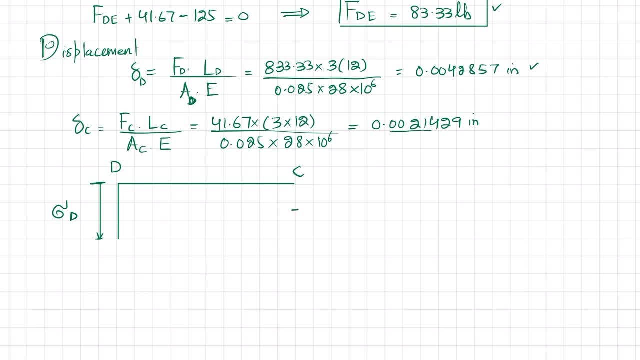 Of this. so you can take it like this: and this displacement is- Let me correct it- This displacement is This one And this displacement is Del C. So you can see from this diagram Now that If I plot, if I exceed it using dotted line, you will see that this is the same as del C and this del- this is equal to this distance- will be equal to 0.0021429, while del D is 0.0042857.. 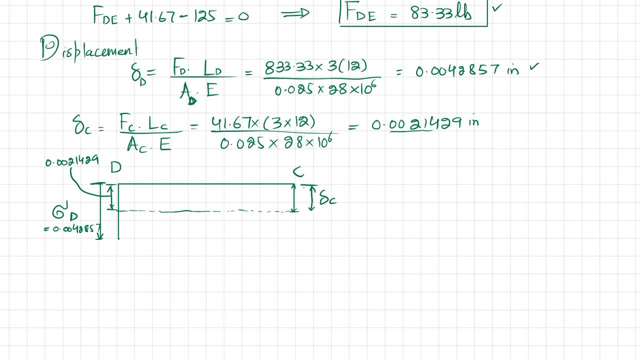 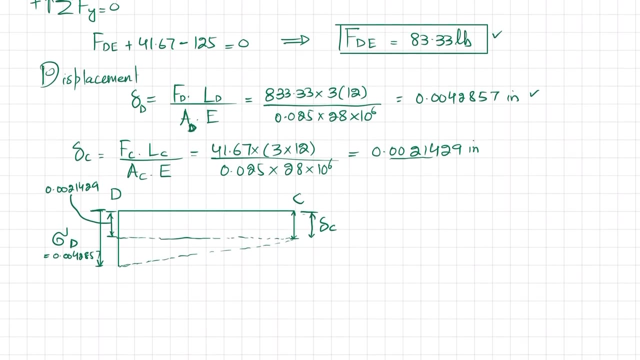 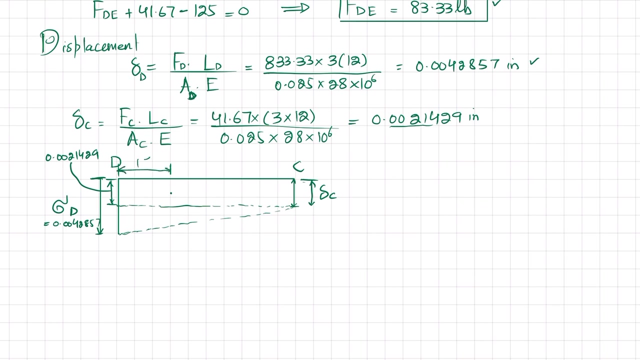 So. So what If I join this point with this There? So We have, we are interested to find out the deflection of this point H. So let this H point is at a distance of one feet Here. this is one feet and this remaining is: 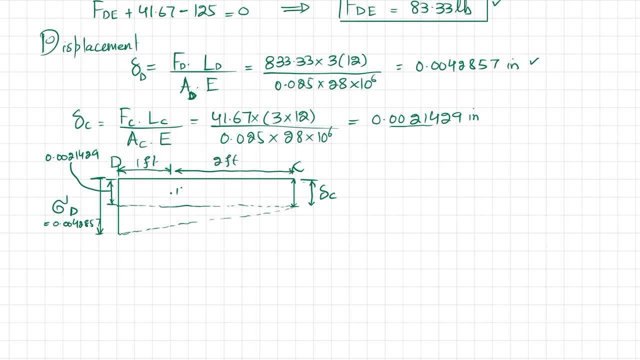 To heat. And this, And this was your original point, Sorry, not this point. This point is your edge point. Let me correct it. This is two feet. This is your point. edge Clear Now. the edge point will cover this displacement. 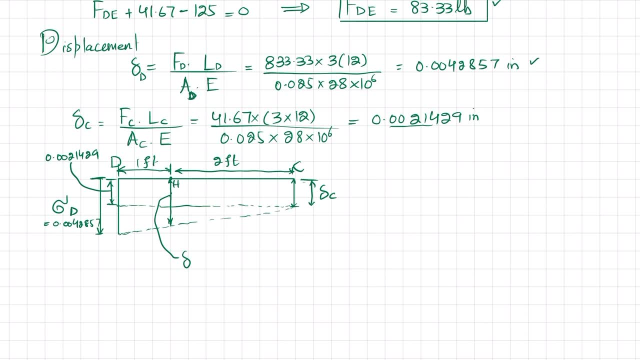 This displacement and this total displacement is del H And this will be equal to Del C, Because this, this distance, is del C And this portion is Del edge dash, Del edge dash. So how you will find this del H dash. 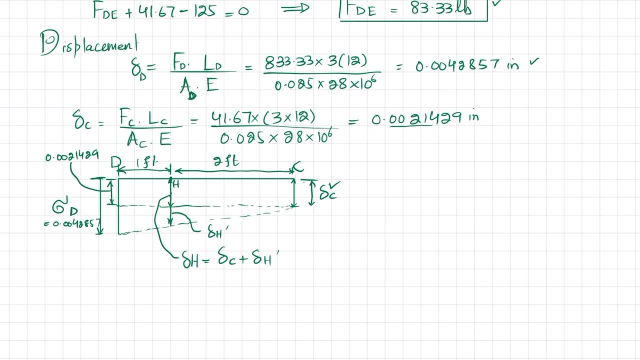 So you can see that. I will show you this If you take this as a right angle triangle There. So this del H, This distance over two feet, Will be Equal to This distance, Which is, Again, this Divide by total three feet. 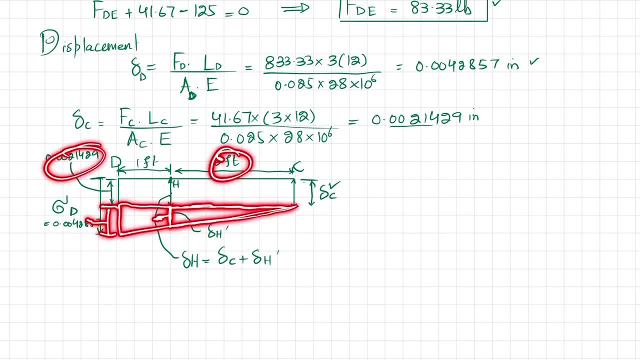 Distance. I will Explain you. We have two similar triangle. One is this one, Clear, And other is This one. So their ratio side, Their side ratios will be Same. So Del H, Dash Over two. 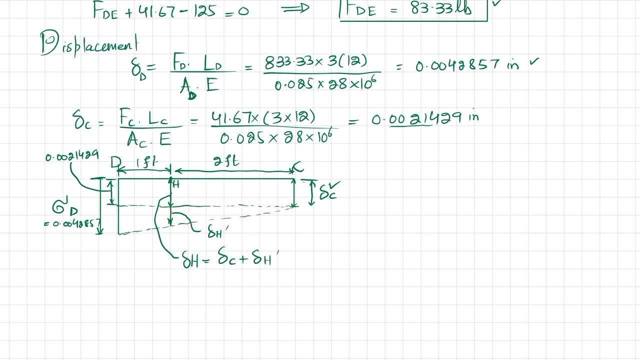 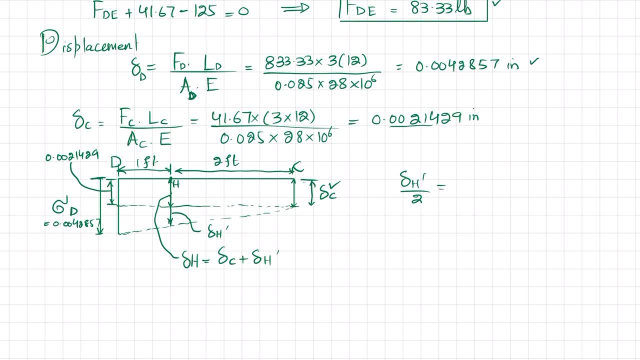 Which is two, Is equal to This Height, Which is Again This Or this, Divide by two, Divide by its Total length, Which is Three feet. I hope It will be Clear. So 0.. 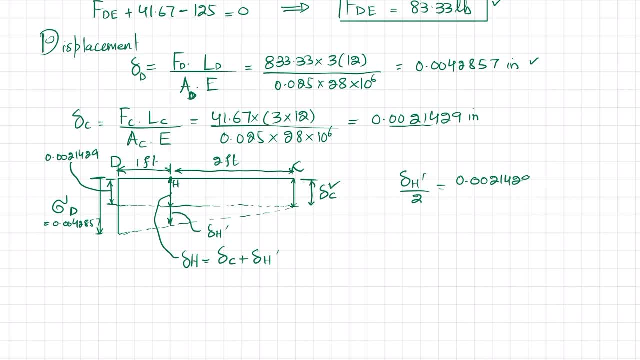 0.. 2021.. 4029.. Divide By 3 feet, So From Here You will get Del H. Dash Will be Equal to 0.. 001.. 4. 286.. 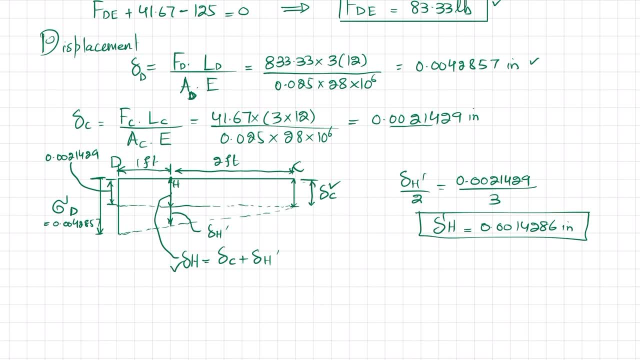 Inch. Okay, So total- We know That total E Rhode Hirth Displacement of Point Edge Is equal To D SEA 29 plus del h dash, so 0.0014286. so you will get total displacement of point h. 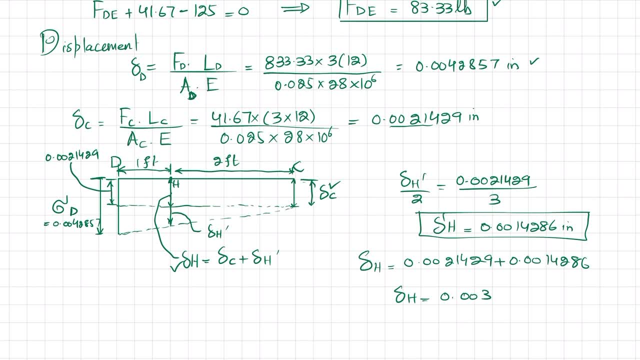 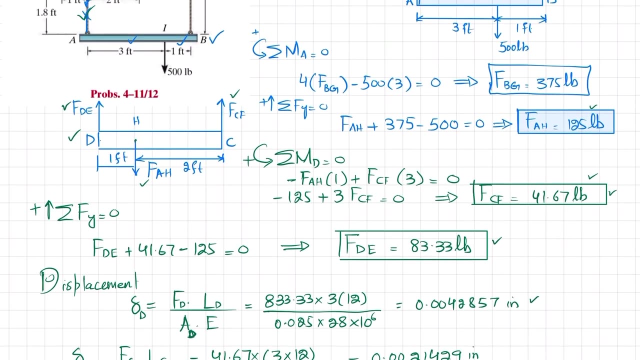 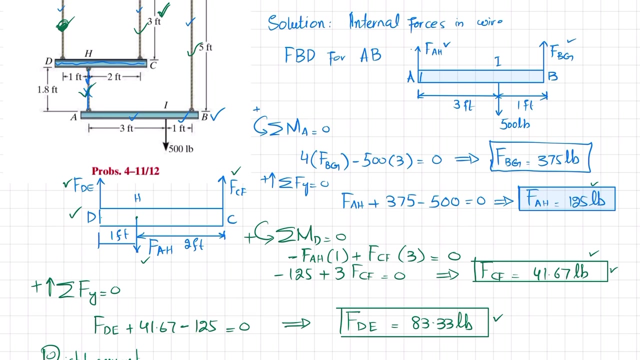 comes out to be 0.0035714 inch. okay, so this was for member uh dc. clear, we will move and we will find that this because, now you can see, this point a is attached with this h, so this point a will also move downward, so we will. 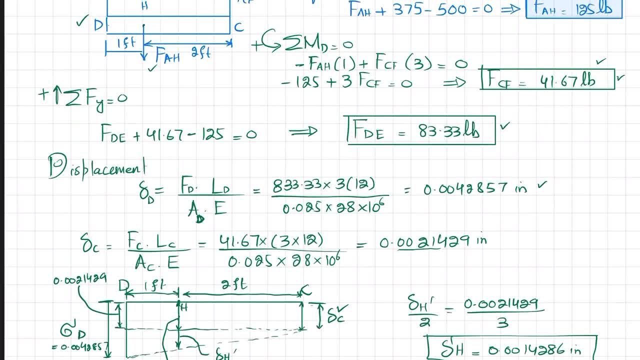 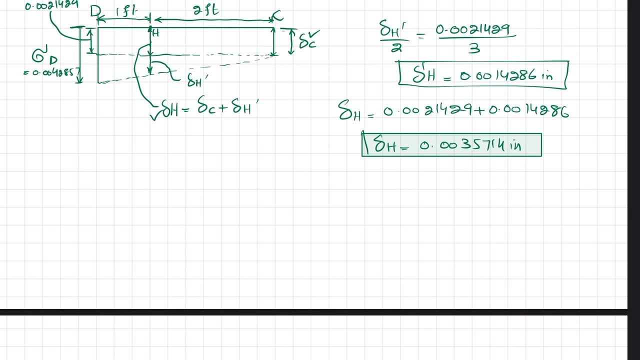 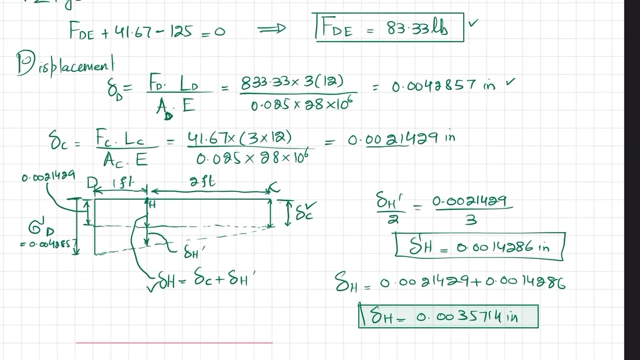 our focus will be now on this beam. so let's draw this beam and also: uh, you also. we will find that. so let this was the. i will choose another color. let this was the beam here. this is point a clear, and we will find displacement. okay. so before that, i will go. 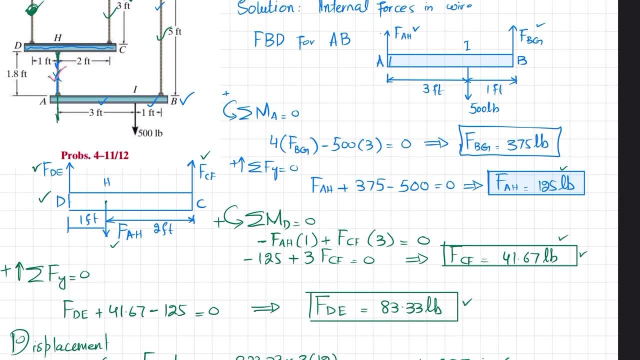 and we will find the elongation displacement in this wire, ah, and this wire master exceptions. ok, let's move on. when we go for the depends on the 모습 r three. so we will, um, we will find a, c, ah, and we will find that if in the above lower left corner, if there is some, 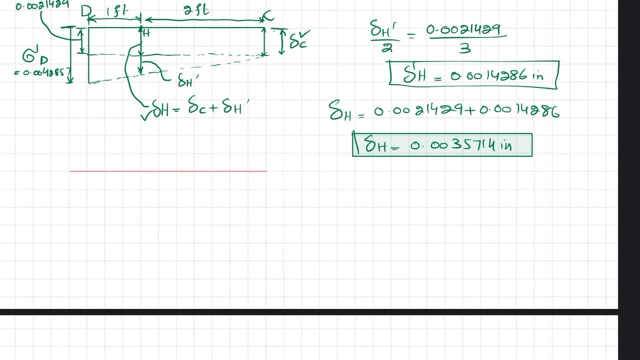 location of b Comme des do we have a cm and we will have an ah in the middle and there is only this wire vegetables in one side as the fashion line. so let's find another color. let's do that So how we will find displacement. So displacement of AH wire will be equal to FAH into length of AH, divided by area of AH into E. 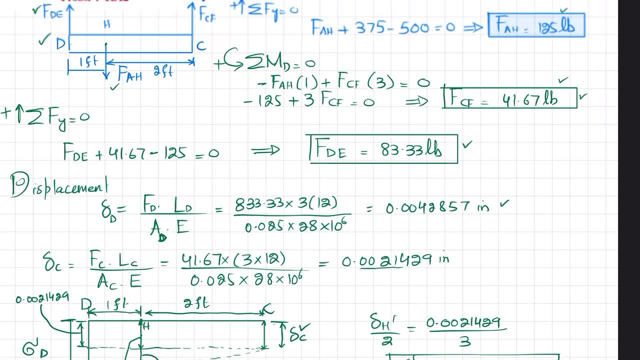 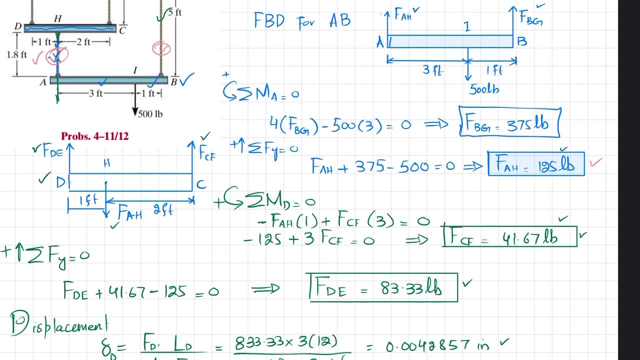 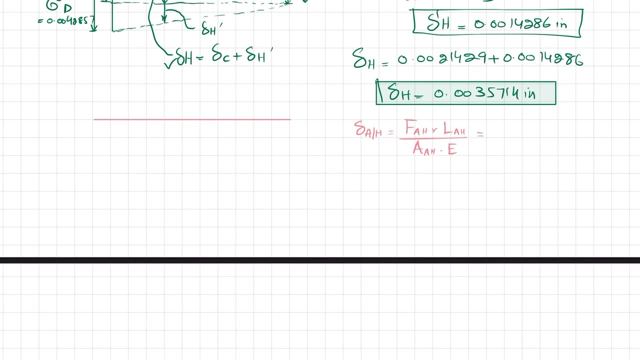 So FAH, which we calculated above. FAH is 125 pounds, length is 1.8 feet. So let me put the values. FAH is 125 pounds, length was 1.8 feet, So 1.8 into 12 will be converted into inch area is 0.025.. 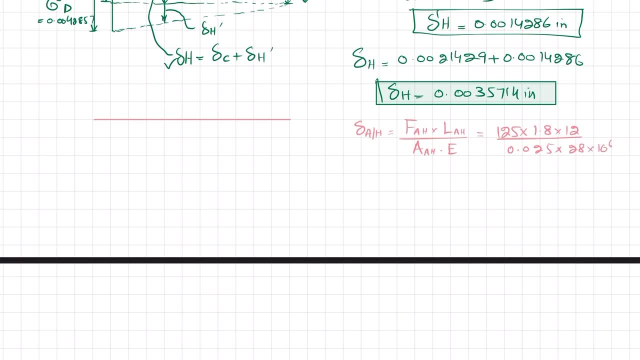 Into E, which is 28, into 10, raised to power 6.. So displacement of point A with respect to H will be equal to 0.0038571 inch inch. Okay, so this is displacement of point AH. Now, total displacement of point A is displacement of point H. 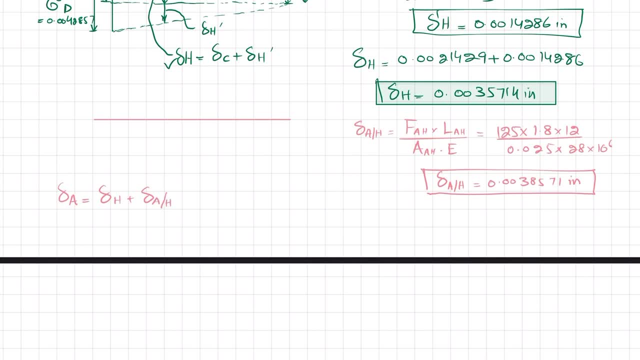 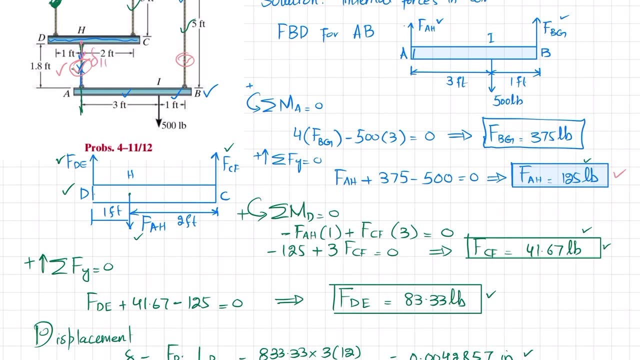 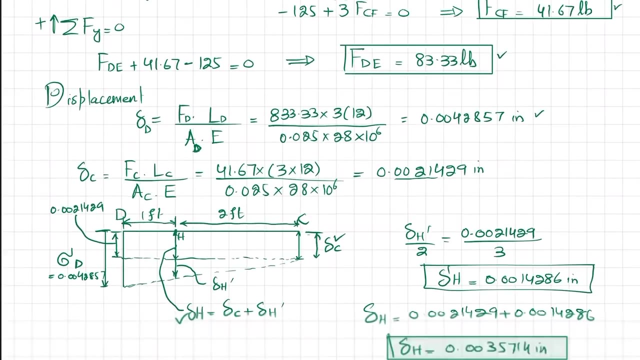 H plus displacement of point A, slash H. I will explain, You can see this point H will move downward, clear. So this displacement is point H and this displacement of point A with respect to H. So total displacement will be this one, point A. 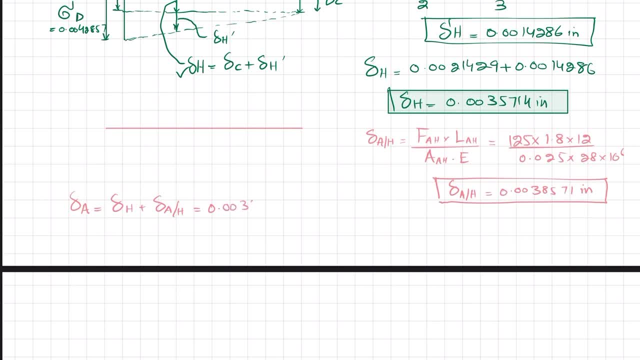 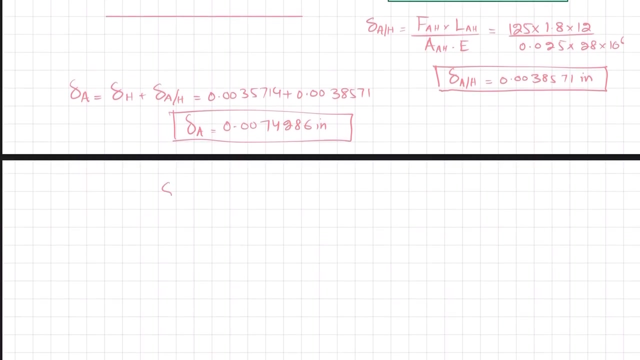 So you can put the value 0.0035714 plus 0.0038571.. And that will be displacement of total. displacement of point A is 0.007486 inch. Similarly, displacement in wire B is equal to FBG into LBG divided by area, BG into E. 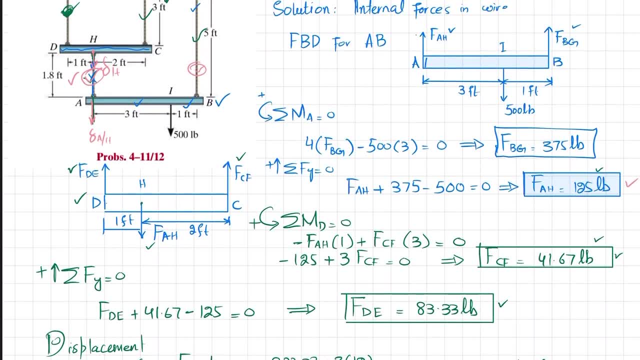 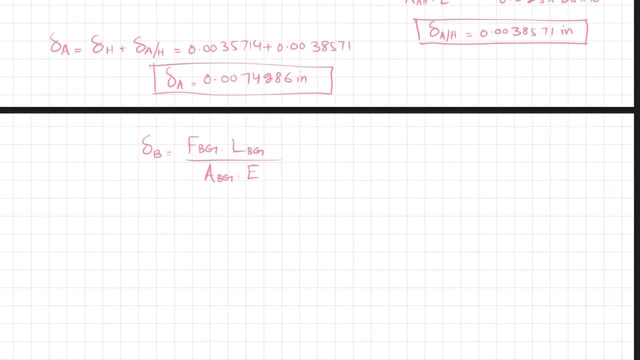 So FBG is 378.. Length is 5 feet So you can put the value. So FBG is 375 pounds. Length is 5 feet. So 5 into 12 will convert it into inch Area is 0.0025 into E, is 28 into 10, raised to power 6.. 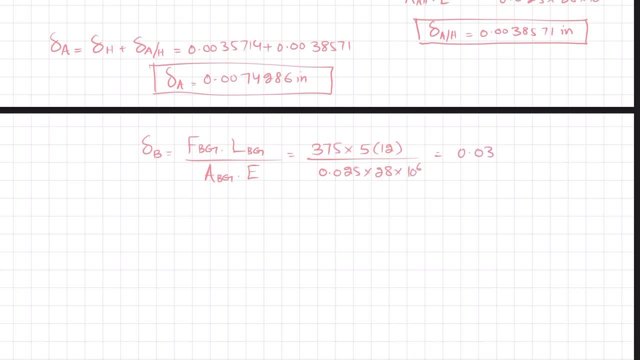 So from here you will get 0.03.. 2,, 1,, 4,, 2,, 8 inch. Now this is the displacement of point B. So if I draw the beam, this was initial the beam. This is your point A. 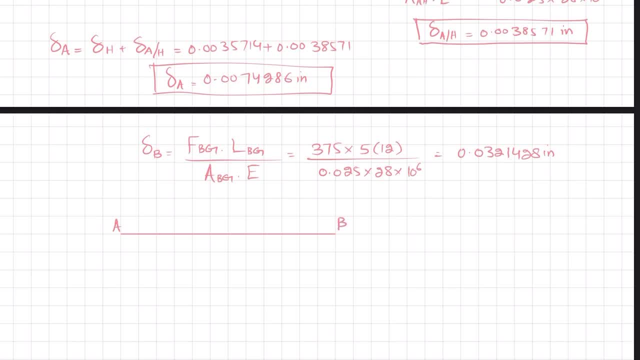 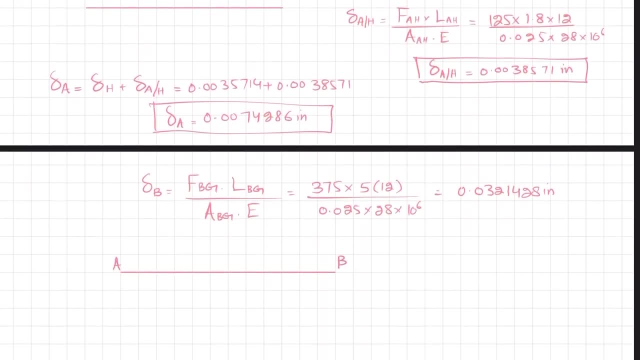 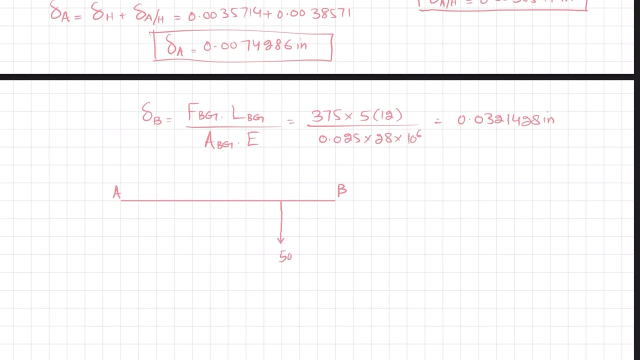 This is your point B. At a distance of 1 feet from point B, there is a load of 500 pounds. So at a distance of 1 feet, there is a load of 500 pounds, 500 pounds. Clear now what we have calculated. displacement of point. 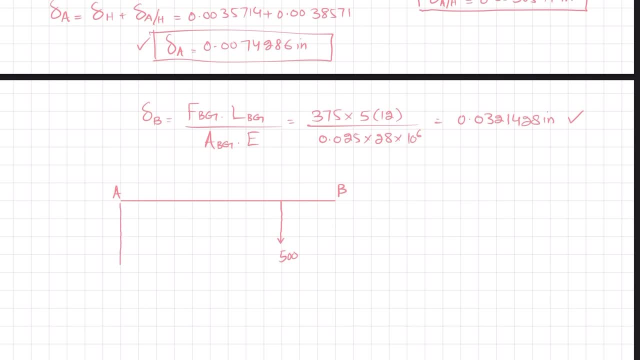 A and this is displacement of point B. It means displacement of point A is larger. So let, this is the displacement of point A And this is the displacement of point B. There I will show. this is your displacement of point B, which is 0.03214. 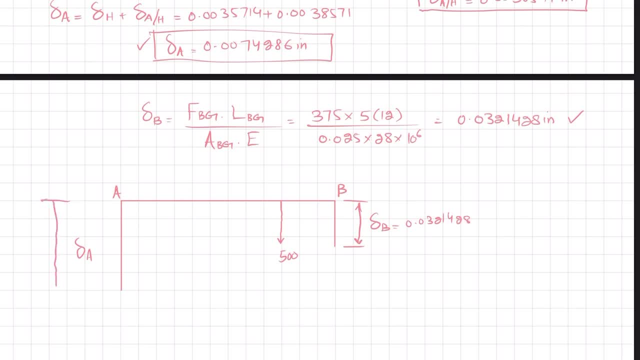 28. this is the displacement of point a, which is 0.0074286 clear and due to this load p, this distance is one feet and this remaining distance from a to B is three feet. so I will remove this force temporarily because we know that at this point we have a load of. I will show. 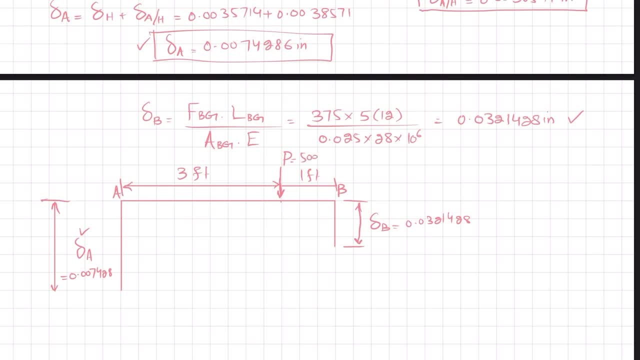 it over here. P is equal to 500 pound. so you can see that if I draw a horizontal dotted line, so at this point this is same as del B. and if I connect this point with this, if I draw a straight line, so you can see that. 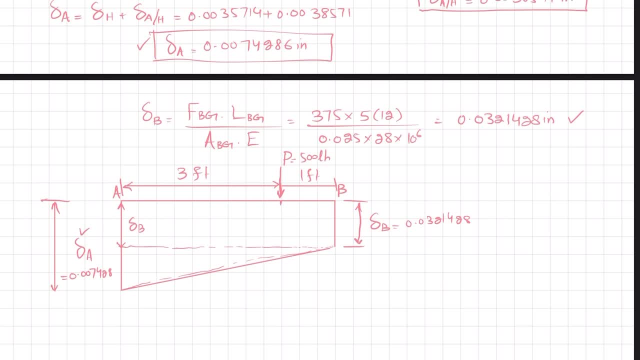 this point. this is the total. this is the total. displacement due to load P is equal to 500 pounds. so this will be equal to 500 pounds. so this is del B and this is sin白 and this will be equal to this del B. from this to this, this is del B and this is Del L' and let the total 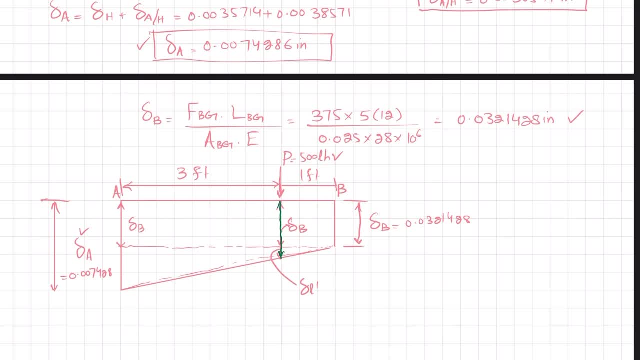 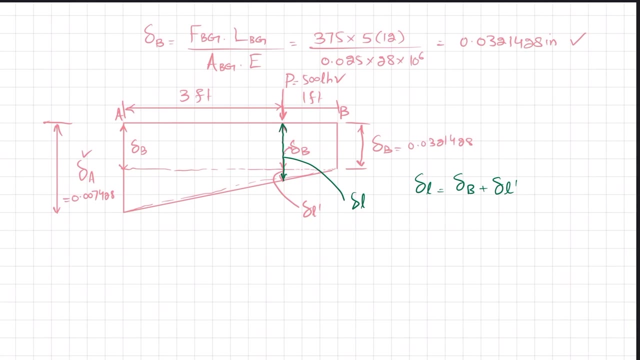 displacement from here to here. this is equal to del by L, so del K is equal to Del B plus del l' and we find that times S≛ 0. buldau. so again you can see that we have two similar triangle. one is this triangle. 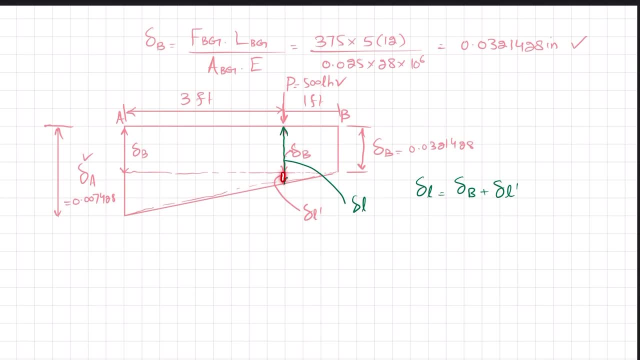 and the other one is this triangle: okay, so by using similar triangle we will find this. so Sigma L del L' threshold, because this is at a distance of three fields del over three is equal to 0.0247143 over 4. okay, so i have. what i have drawn is three feet, three feet at point b, at point a, so point a is one feet. 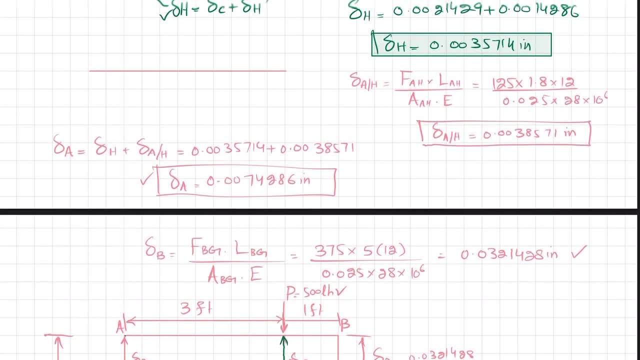 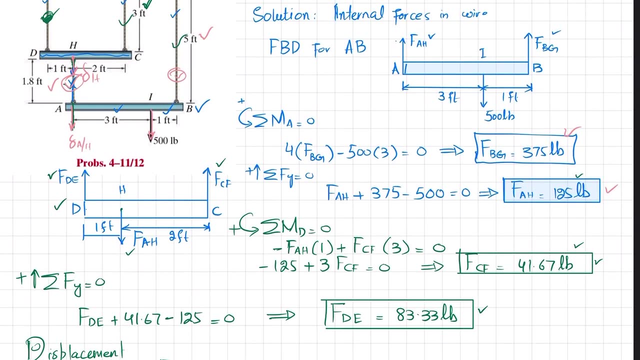 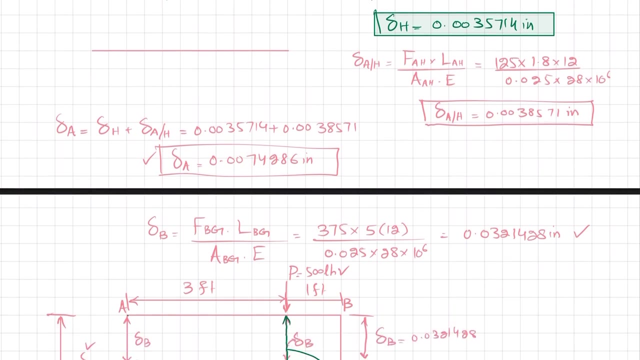 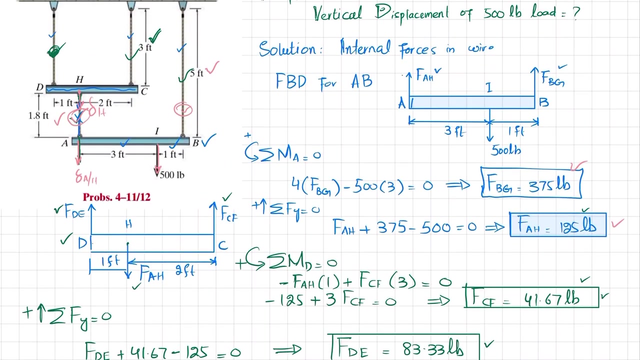 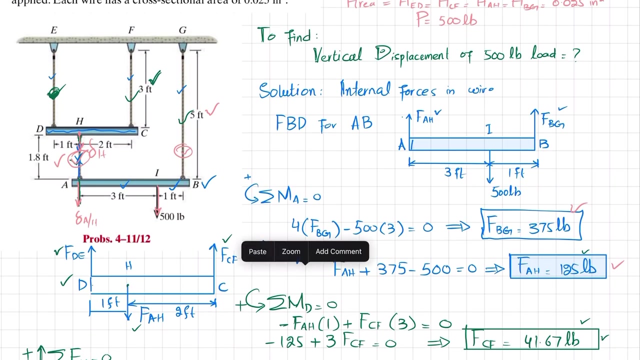 three feet. let me check it. point a is this one, a, h, a is this one and b is this one due to load. so point a, we have this and b, we have this. point a is a distance, of b is one feet and this is this is. 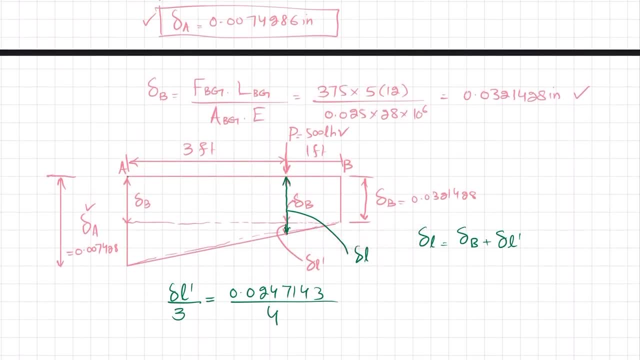 three feet, okay, so, so del l dash over this three feet. one feet is equal to this. over total l. okay, so del l over three feet is equal to okay, so del l dash over perpendicular distance over. here is i have. then. this is point b. at point b we have 0.034. okay, so i find found the mistake. the mistake is in this. 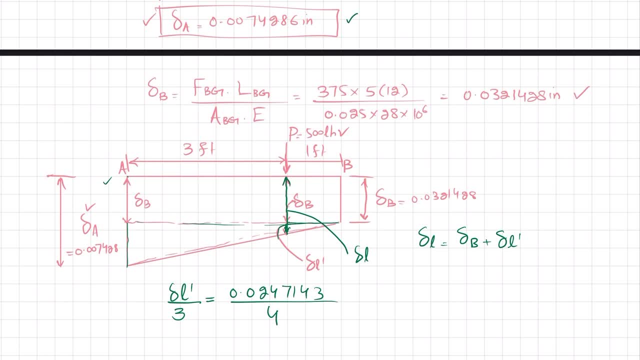 diagram so you can see del a is small and del b is larger. so we will modify this diagram again, so it will take time. let me correct it in this way: you will have a clear idea, understanding about this and you will learn it. okay. so this is your sigma. 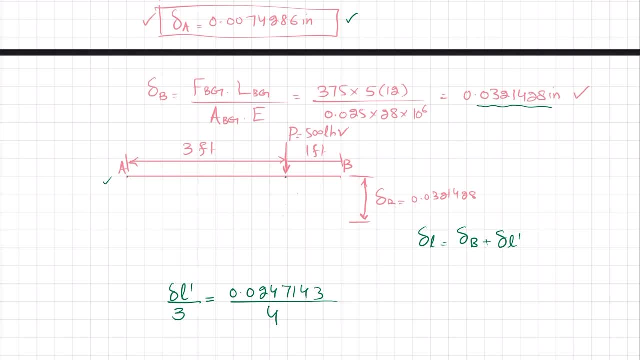 this is your sigma b, clear. this is your del b, sorry del b. and del a is 0.05. let's say this is your del b. this is a very small value and this is a del, sorry a, and that is equal to 0.0007428 and that is equal to 0 point, 0.0007428. 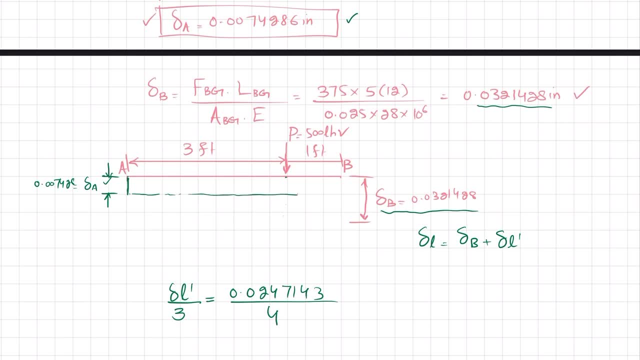 Thank You too. so if you draw horizontal line so you can see that in this portion this will to your and i will slowly draw all stomach then concretize the long line, so the distance line that we have between the dih4 line, point b and amaligh milk paper on the point division length.